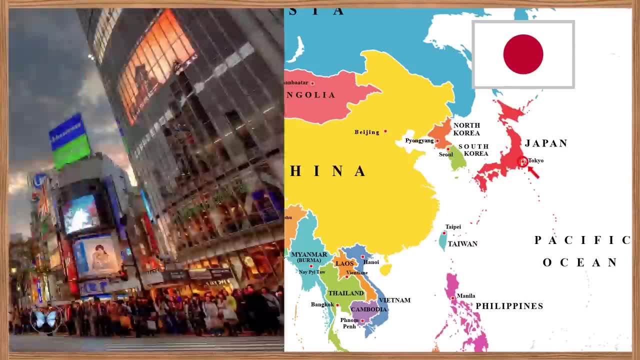 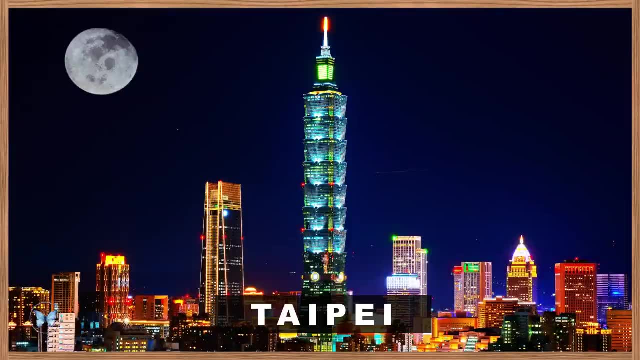 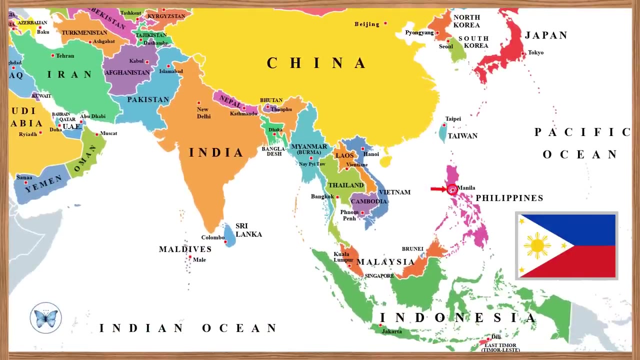 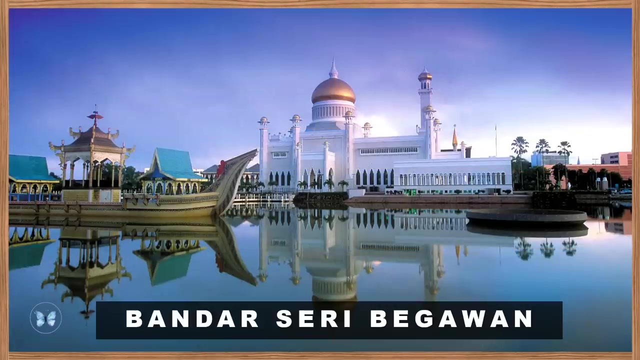 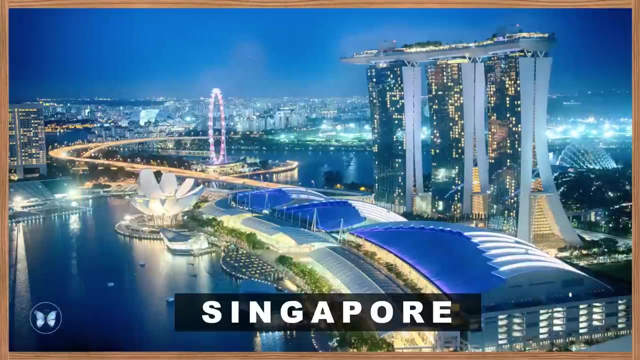 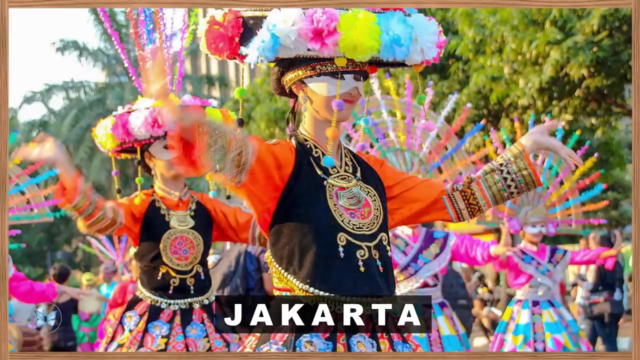 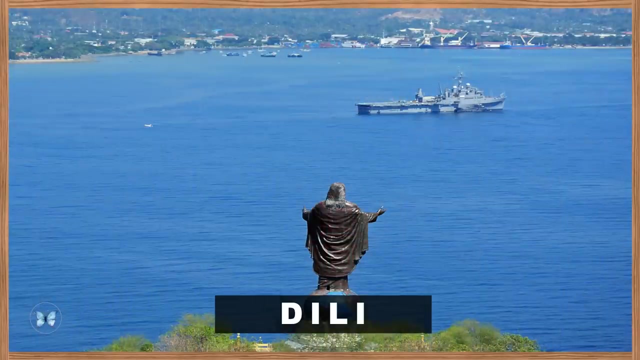 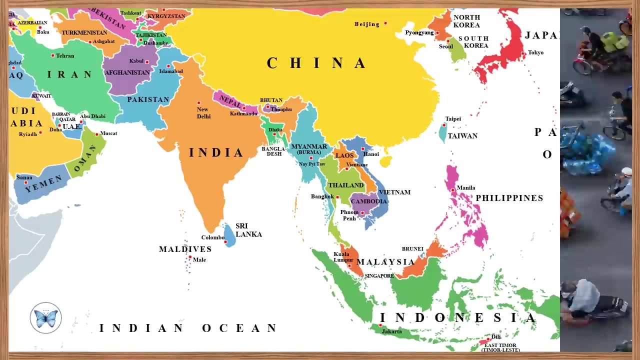 Japan, Tokyo, Taiwan, Taipei, Singapore, The Philippines, Manila, Malaysia, Kuala Lumpur, Brunei, Bunder, Seri Begawan, Singapore, Singapore, Indonesia, Jakarta, East Timor Delhi, Vietnam, Hanoi, Cambodia. 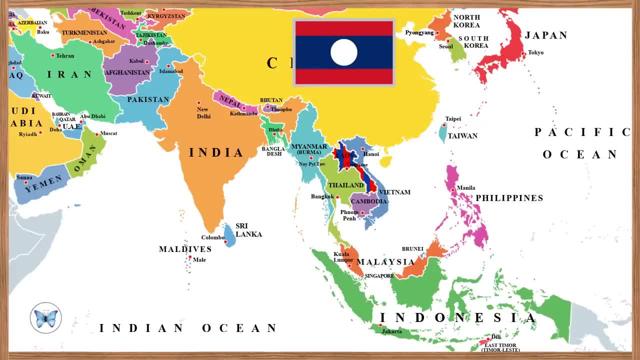 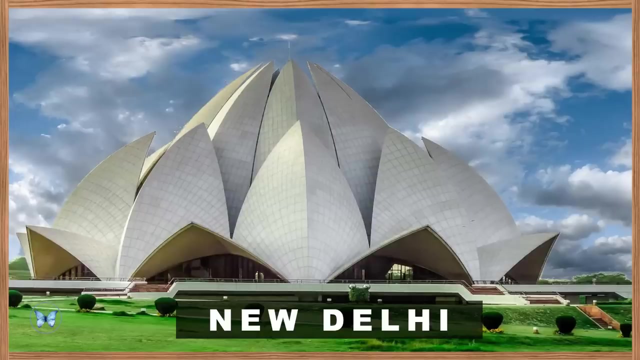 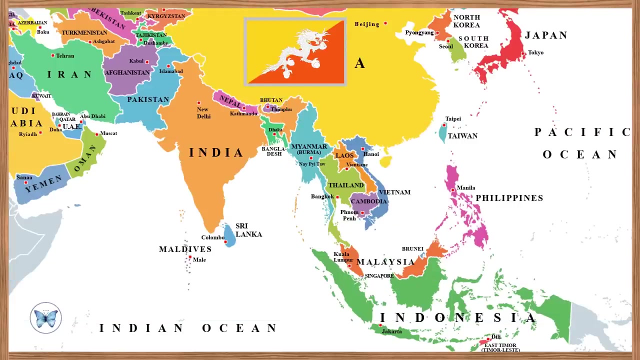 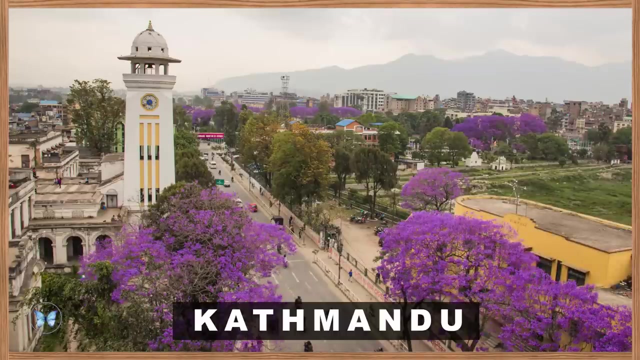 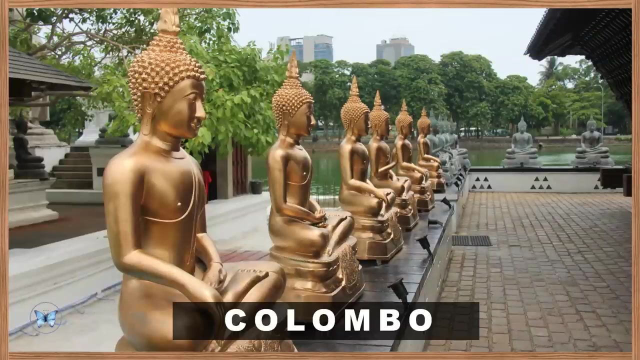 Phnom Penh, Laos Vientiane, Thailand, Bangkok, Myanmar, Nay Pee Thaw, Bangladesh, Dhaka, India, New Delhi, Bhutan, Thimphu, Nepal, Kathmandu, Sri Lanka, Colombo. 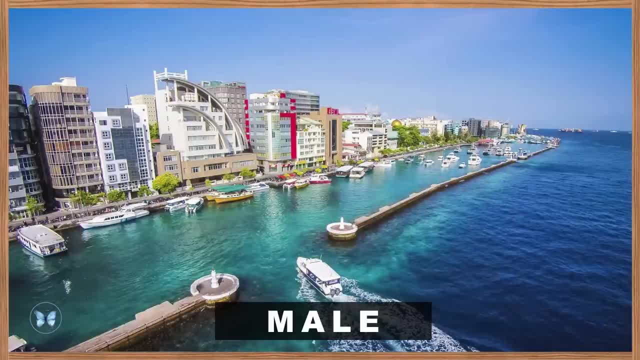 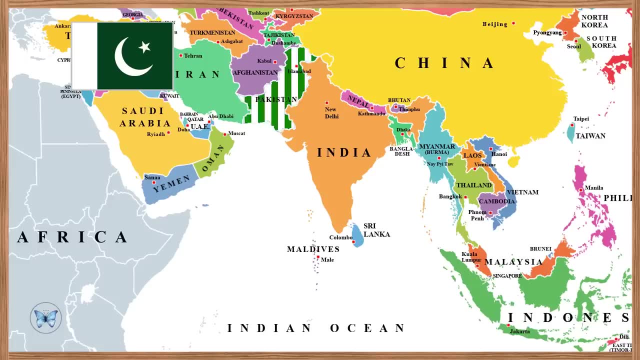 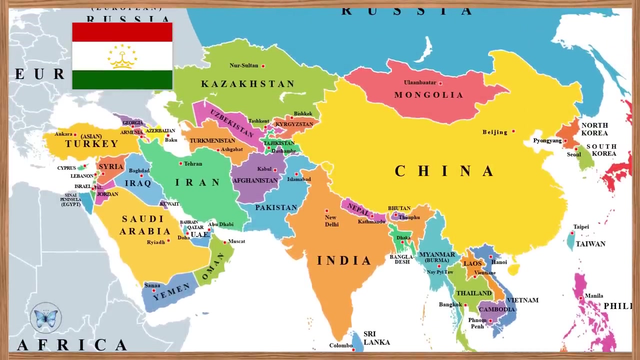 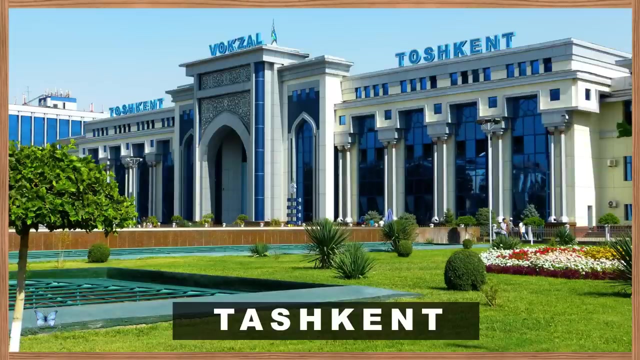 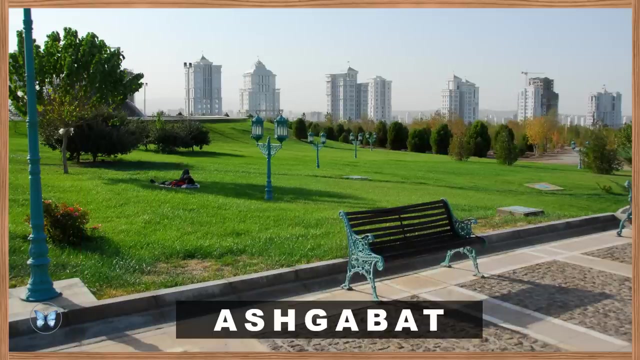 The Maldives, Malay, Pakistan, Islamabad, Afghanistan, Kabul, Tajikistan, Dushanbe, Kyrgyzstan, Bishkek, Kazakhstan, Newer Sultan, Uzbekistan, Tashkent, Turkmenistan, Ashgabat. 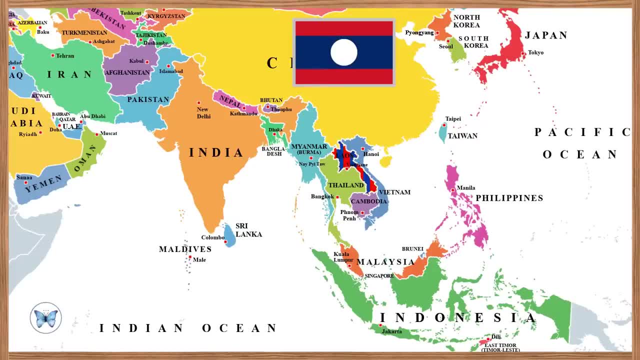 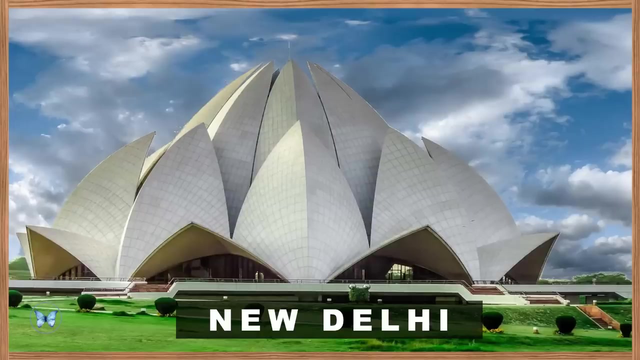 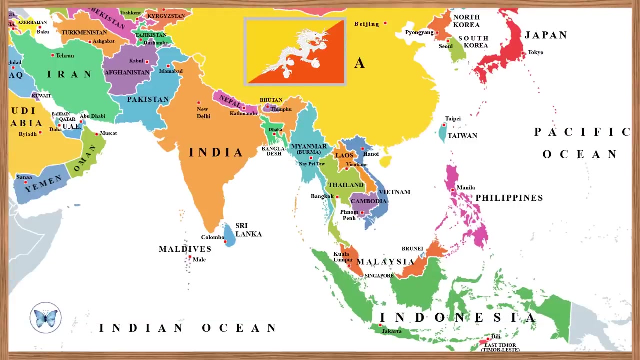 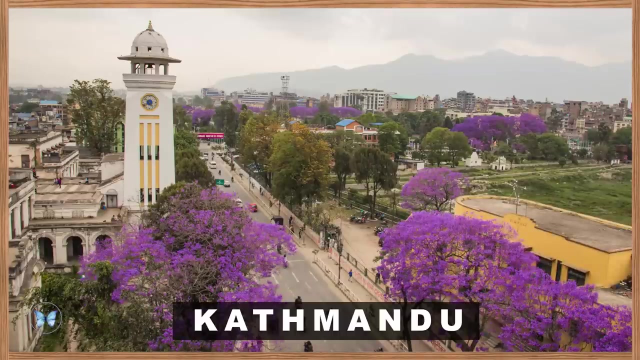 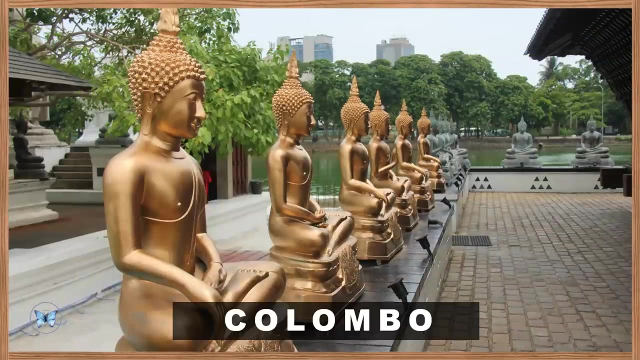 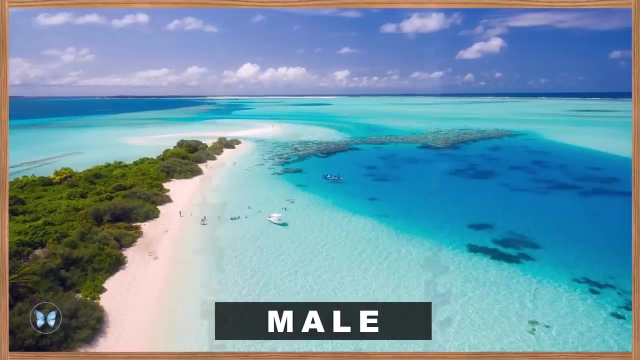 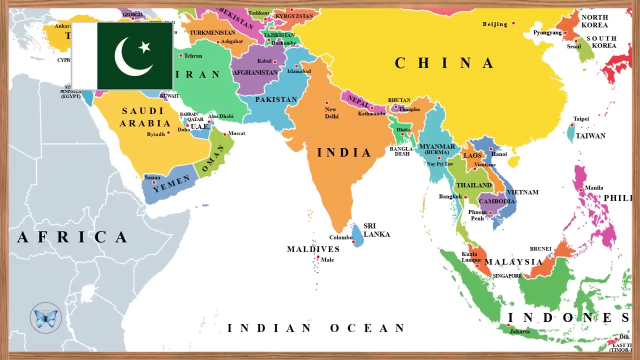 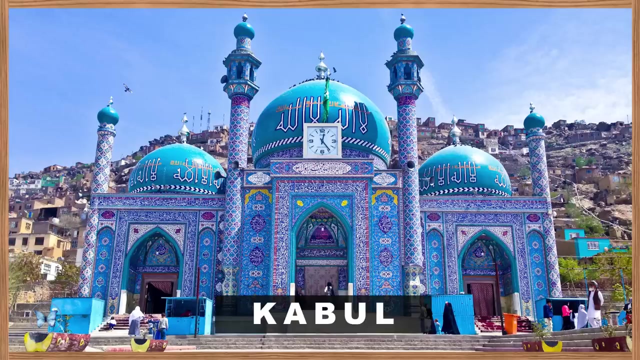 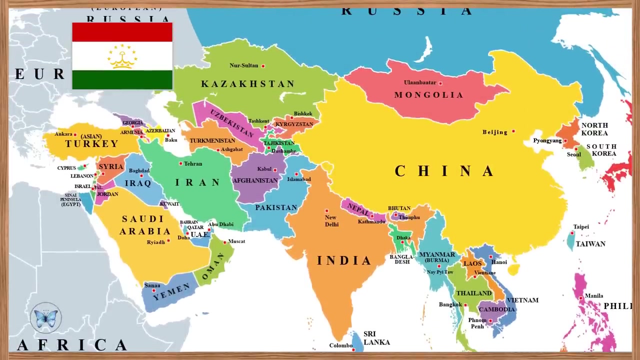 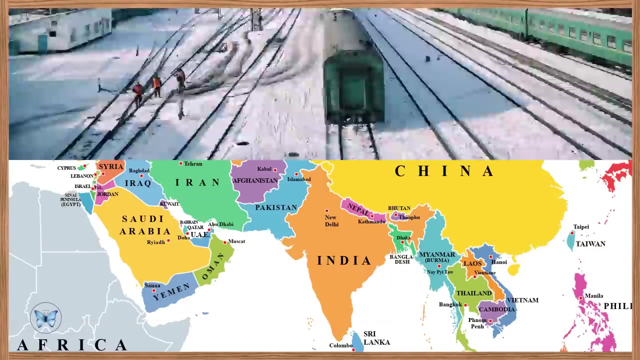 Phnom Penh, Laos Vientiane, Thailand, Bangkok, Myanmar, Nay Pee Thaw, Bangladesh, Dhaka, India, New Delhi, Bhutan, Chennai, Nepal, Islamabad, Afghanistan, Kabul, Tajikistan, Dushanbe, Kyrgyzstan. 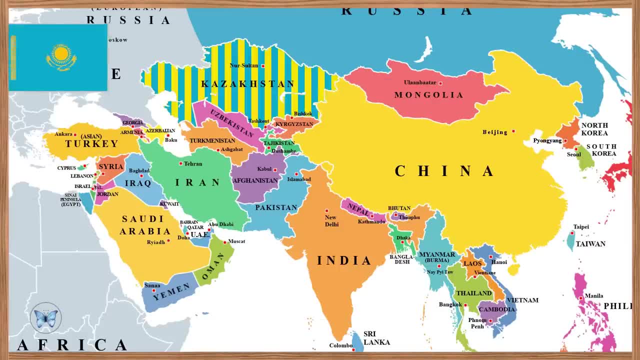 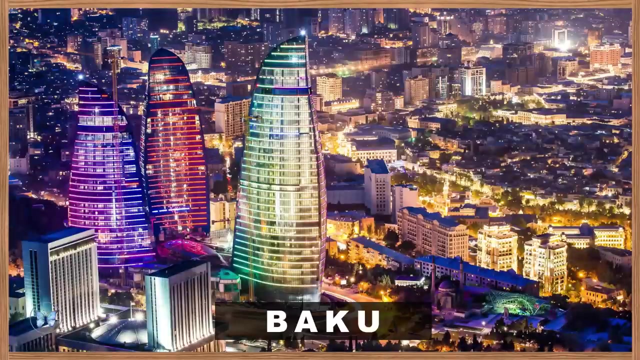 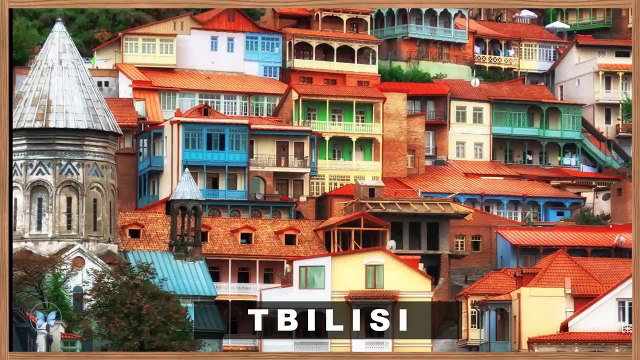 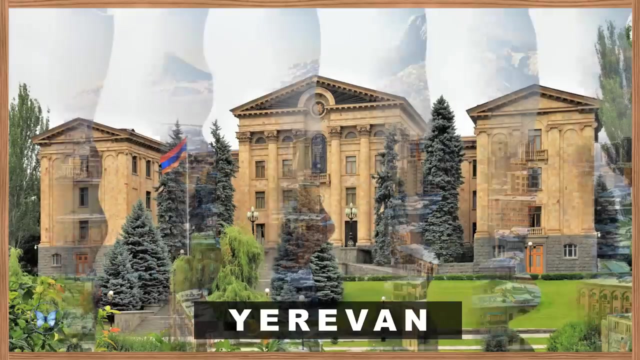 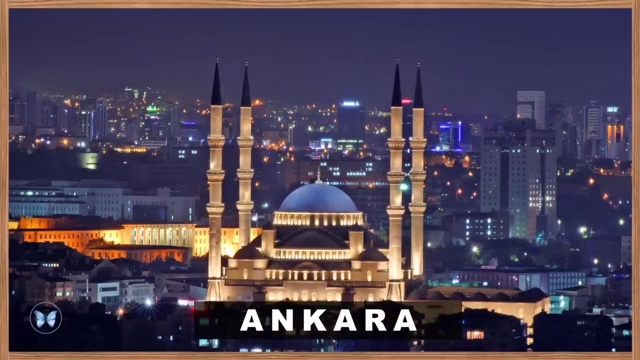 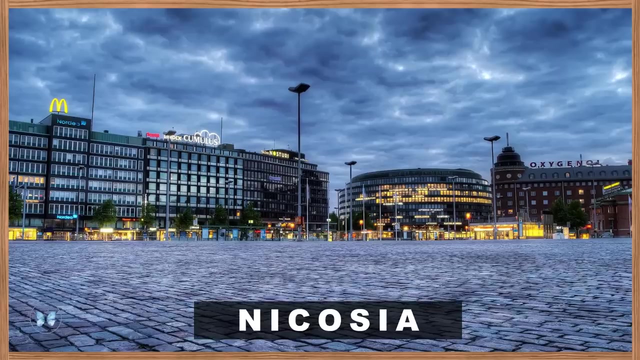 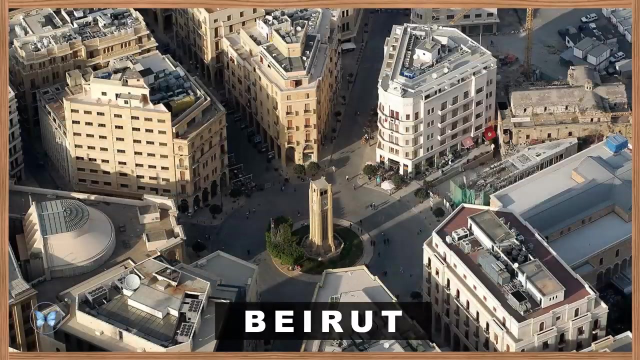 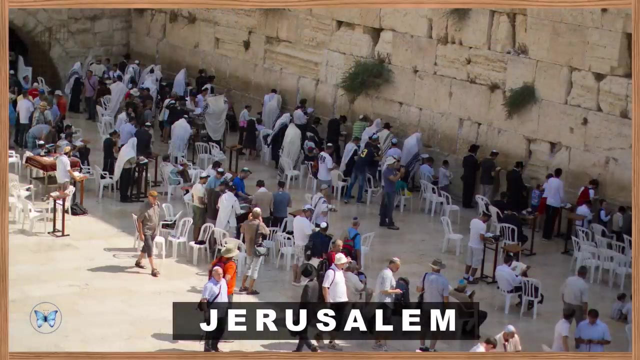 Bishkek, Kazakhstan, Nur Sultan, Uzbekistan, Tashkent, Turkmenistan, Ashgabat, Iran, Tehran, Azerbaijan, Baku, Georgia, Tbilisi, Armenia, Yerevan, Kyrgyzstan, Kyrgyzstan, Kyrgyzstan, Kyrgyzstan, Kyrgyzstan, Kyrgyzstan, Kyrgyzstan. 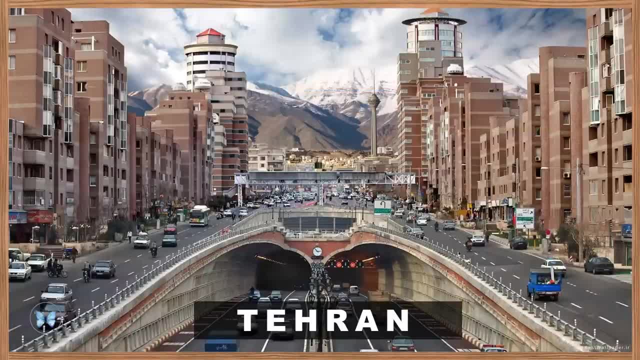 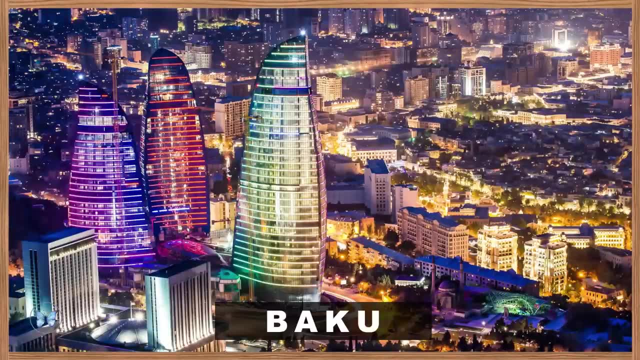 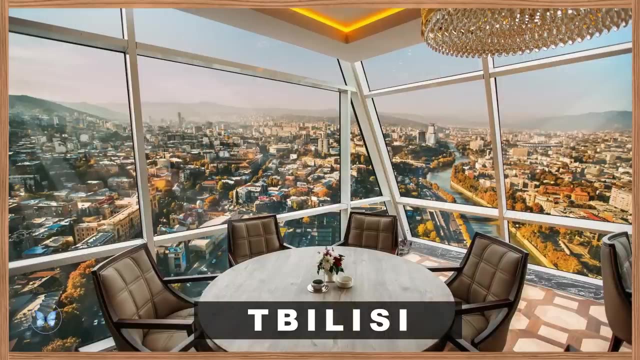 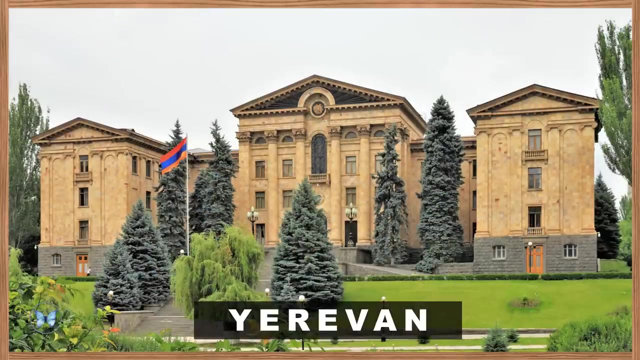 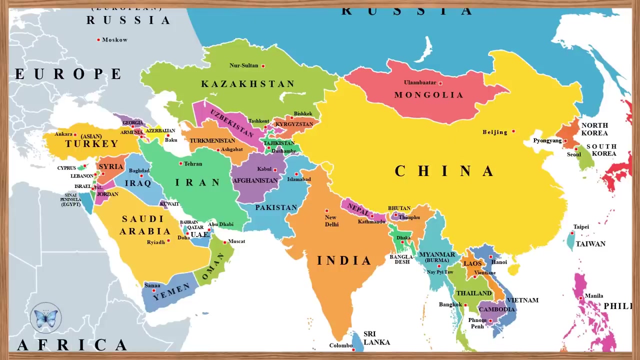 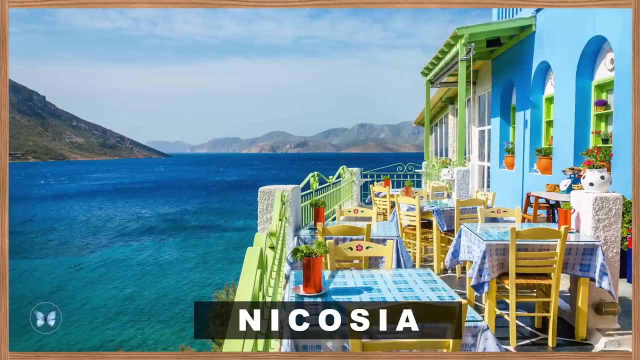 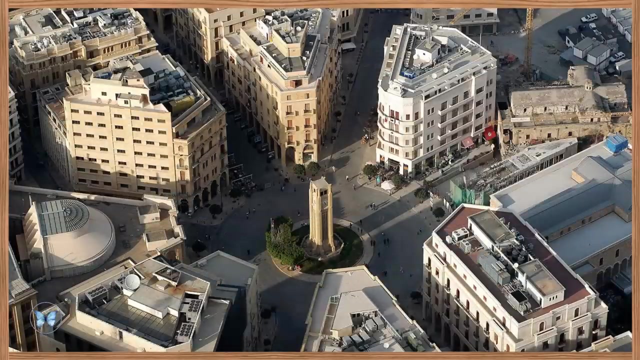 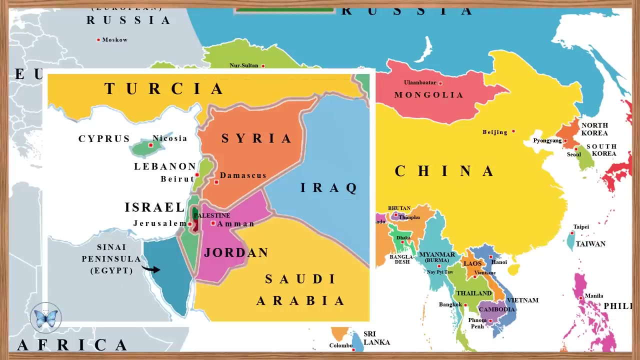 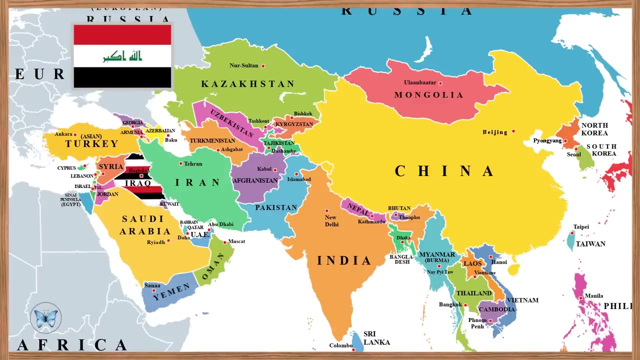 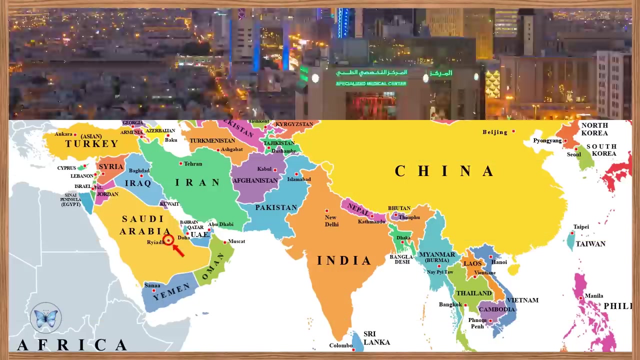 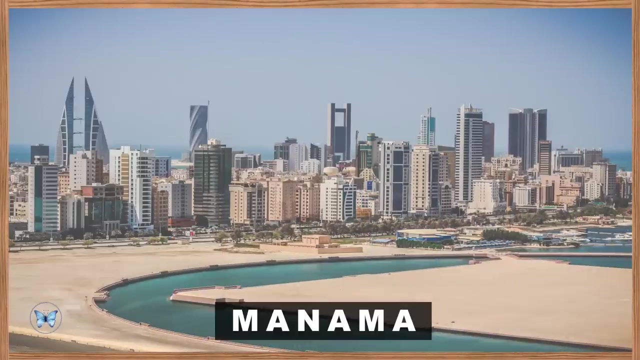 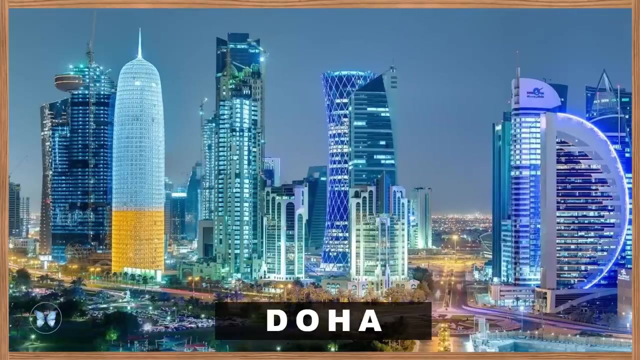 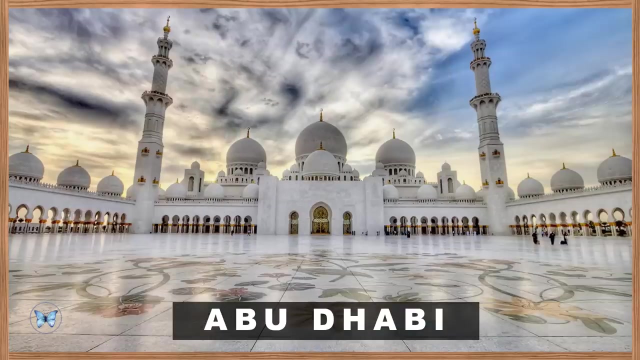 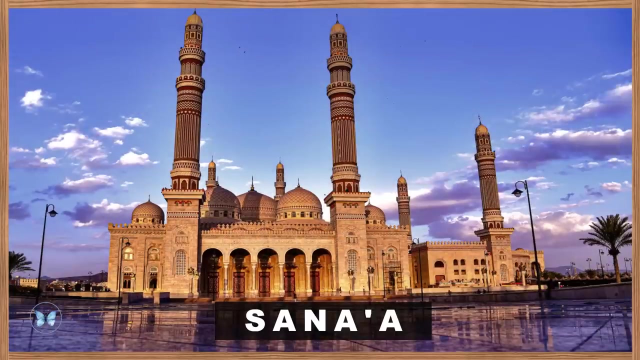 Iran, Tehran, Azerbaijan, Baku, Georgia, Tablisi, Armenia, Yerevan, Pakistan, Congo, Pakistan, Kyrgyzstan, Ukraine, Iraq, Palestine, Pakistan, Qatar, Qatar, Doha, United Arab Emirates, Abu Dhabi, Yemen, Sana'a. 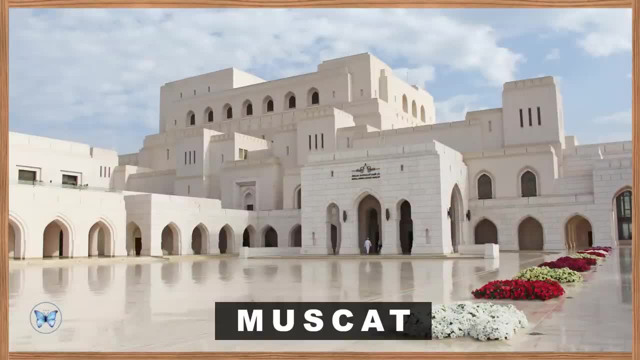 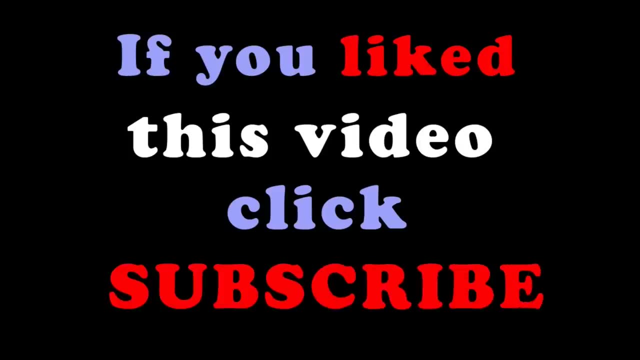 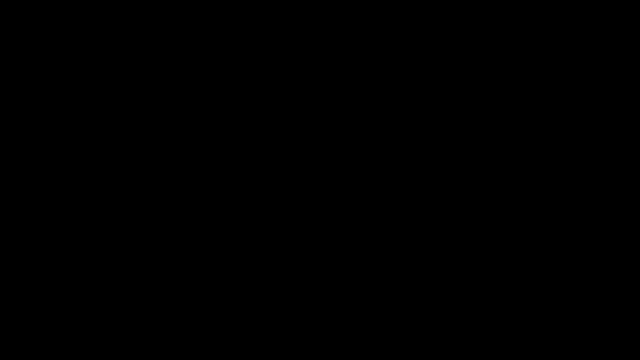 Oman, Muscat, Qatar, Doha. 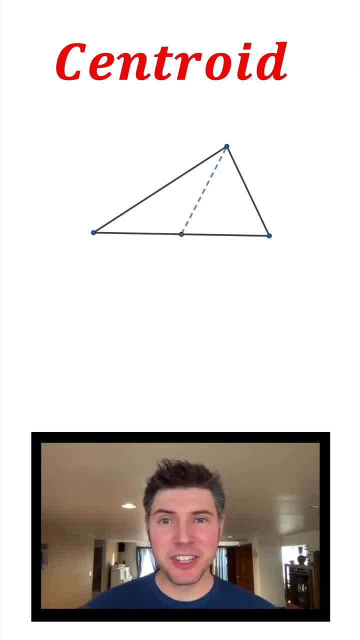 Hey guys, let's talk centroid. So if we take a triangle, bisect one of the sides and connect it to the opposite vertex, this line is called the median. Each triangle has three medians and these three medians always intersect at one point. This point is called 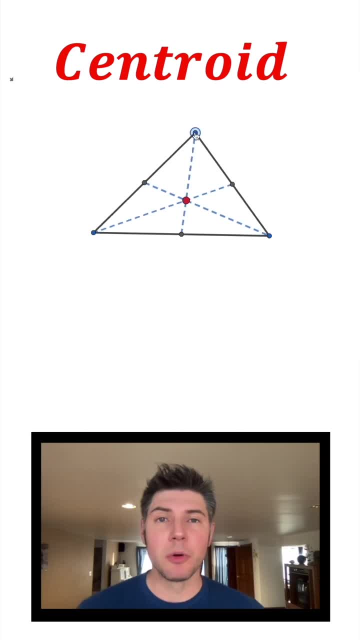 the centroid. Whether the triangle is obtuse, right or acute, the centroid will always be inside. The centroid does something really cool with the medians. It cuts each median into one thirds and two thirds. Another cool thing about the centroid is if you plot this triangle on a 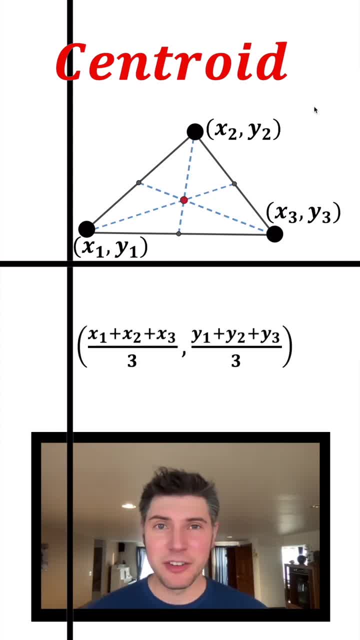 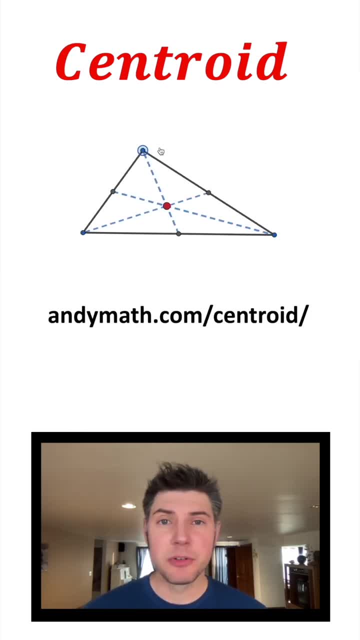 graph and assign plotted points to each vertex. you can very easily find the centroid with this formula right here: You just add up the x values, divide by three, add up the y values, divide by three and you're done. If you guys want to play with this visual on your own, visit andymathcom.